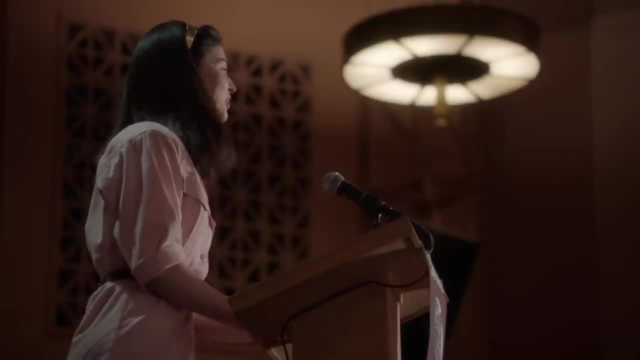 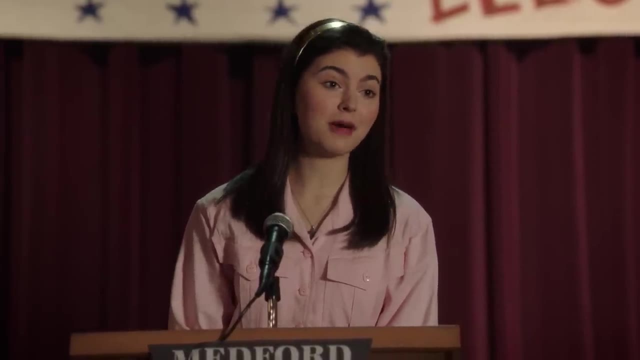 Thank you, Ms McElroy, Principal Peterson, our hard-working teachers and my fellow students. Thank you, Ms McElroy, Principal Peterson, our hard-working teachers and my fellow students. I'm blessed to call so many of you friends. Y'all probably know everything about me. 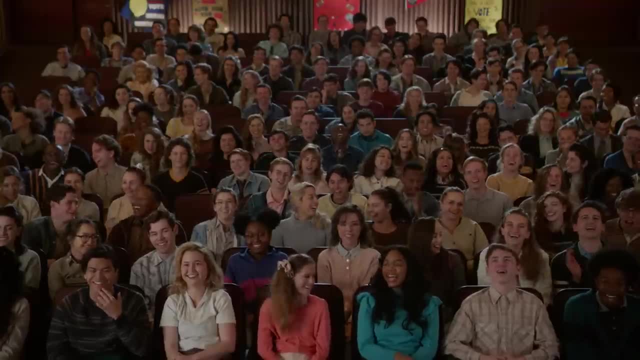 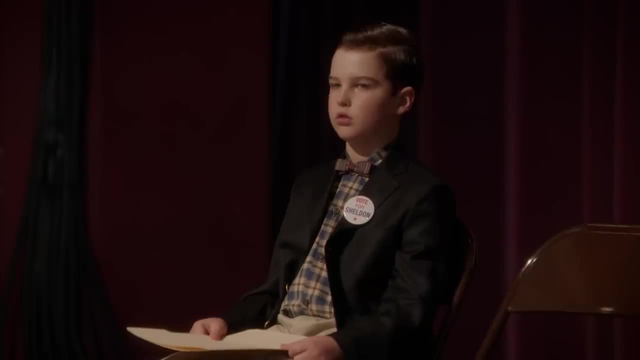 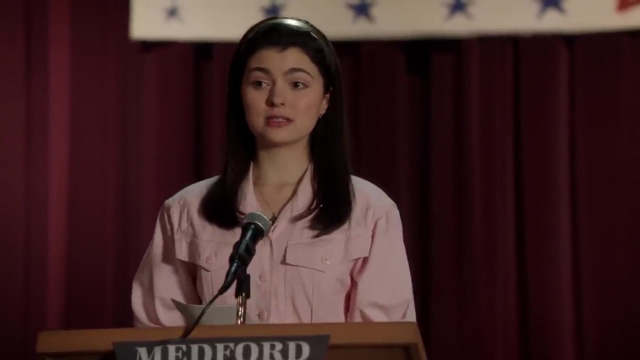 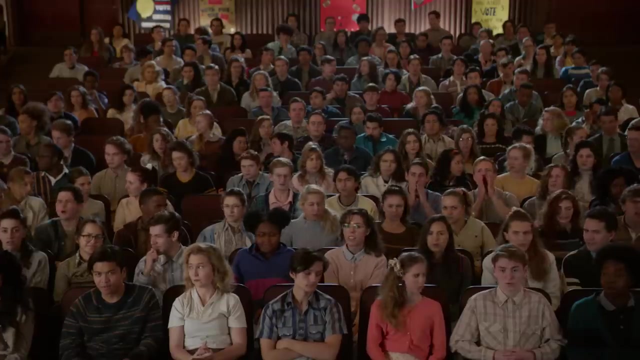 already, Lord knows. I love to talk, So instead of going on about myself, I'd like to talk to you about my opponent. Sheldon Cooper has been lobbying for new science equipment here at Medford High, and while that sounds wonderful, the truth is he thinks our school wastes its money on football. 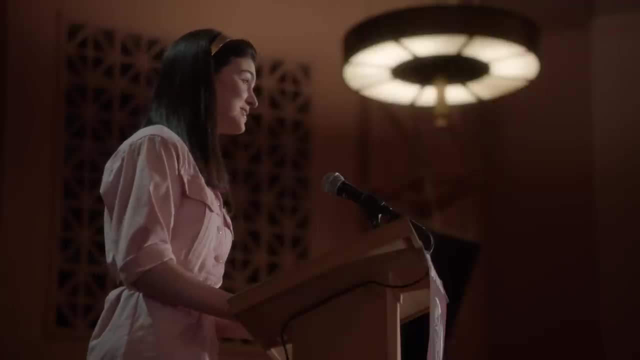 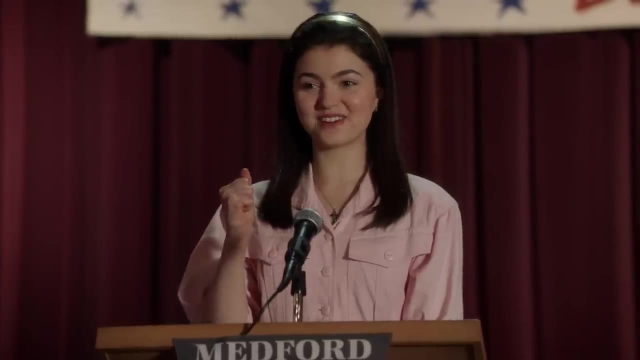 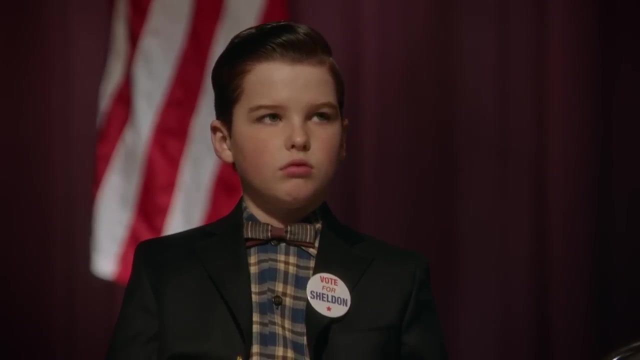 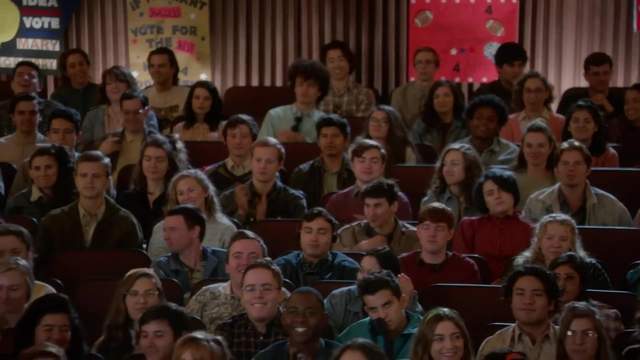 Do we really want a class president who doesn't care about football? I know I'm proud to be a Medford High cheerleader and I love football, But you know the one thing I love more than football- God. Let me tell you another interesting fact. 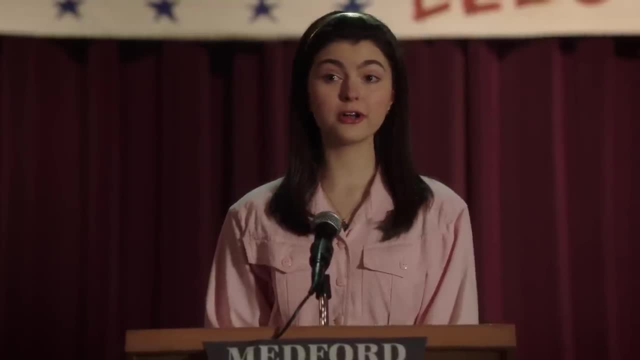 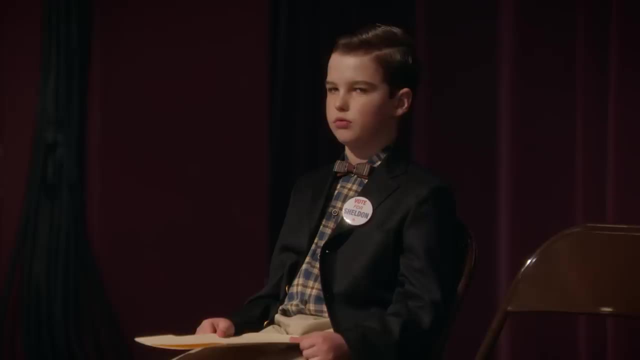 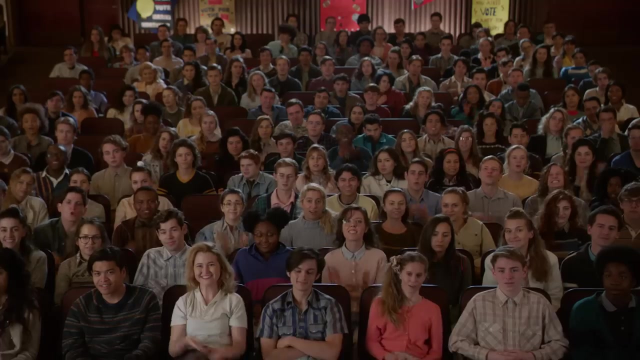 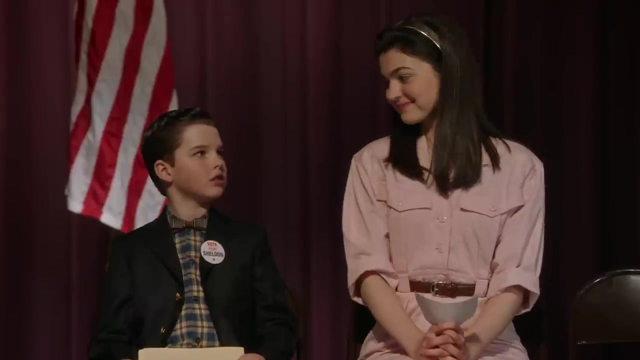 about my opponent. Did you know that Sheldon Cooper is an atheist? That's right. He doesn't believe in God. Just keep that in mind when you cast your vote today. I'm Nell Kavanaugh, Go Wolves, And now please welcome Sheldon Cooper. 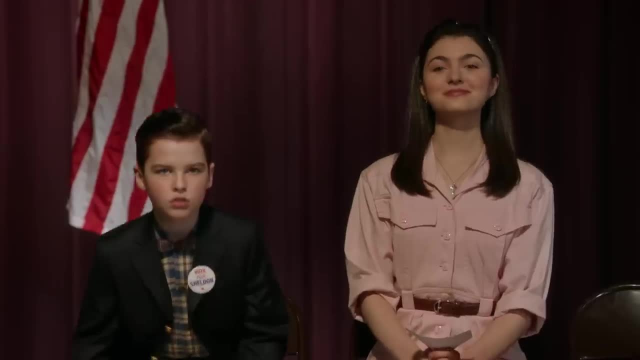 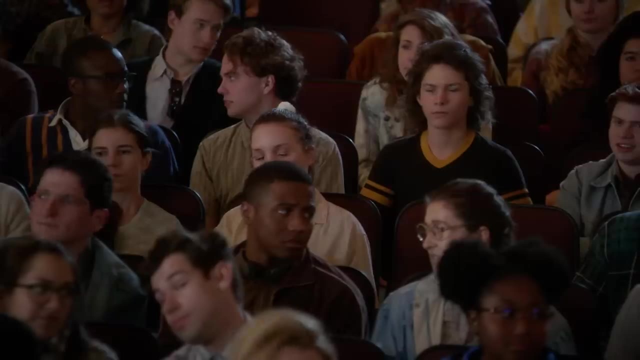 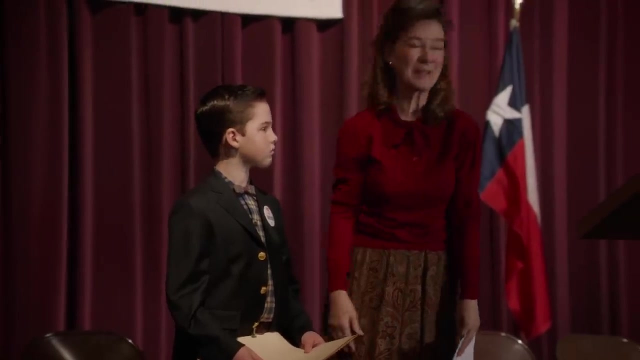 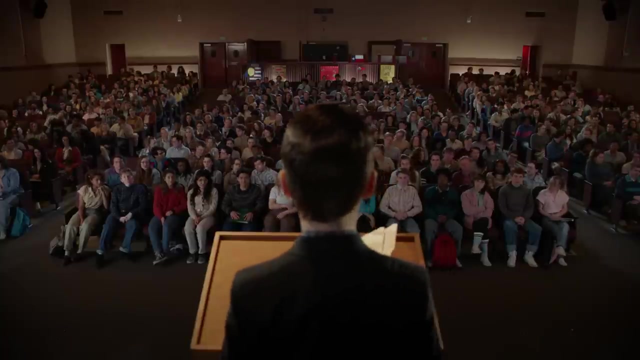 Sheldon Cooper. Open your cards, Close them. Let's do this. There'll be two of them. Sheldon Cooper, Don't let that fall on you if you ran out of the back door. Close your cards, Sheldon. Do not check the books again. 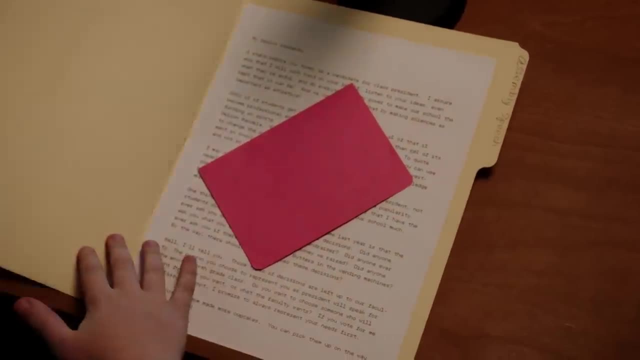 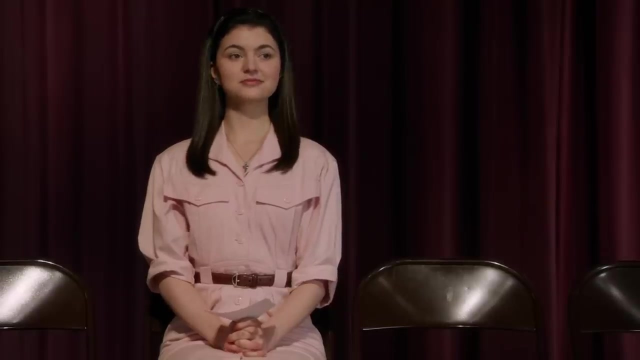 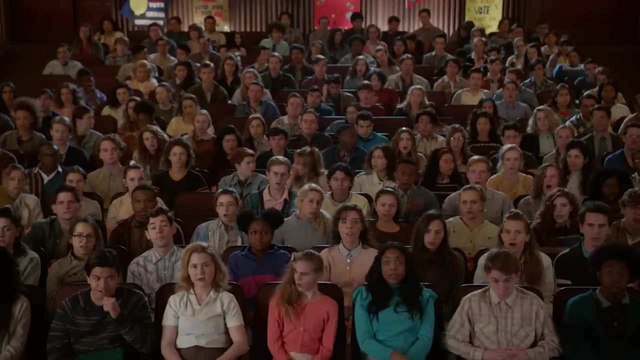 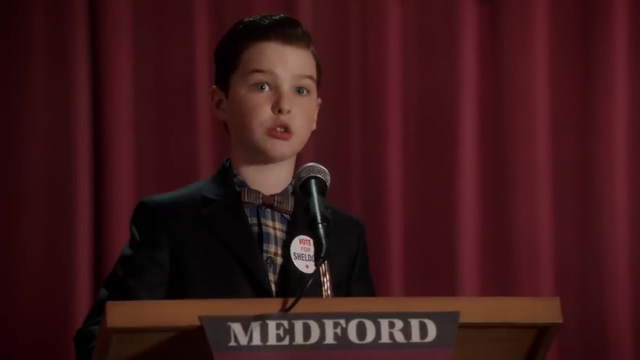 Be hurled on the blindside by an animal. Be your far Commentary on this. No, Kavanaugh is a Yankee. She may love football and she may love God, but she was born in Scarsdale, That's in New York.